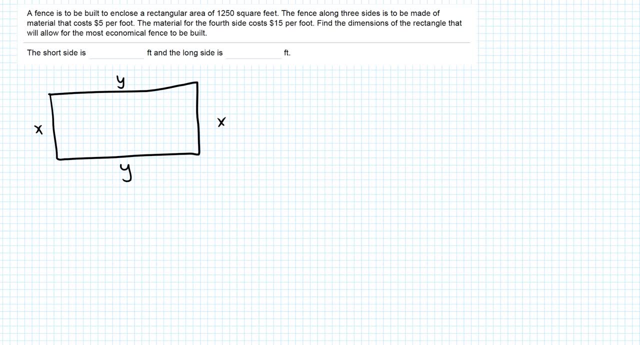 And so they're telling me that it's going to be $5 per foot on three of the sides, $15 per foot on the other side. So $5,, $5,, $5. And $15.. So the cost of making this fence is going to be 5X plus 5Y, plus 5X plus 15Y, So that will give me 10X plus 20Y. I need to figure out what Y is because I can't take a derivative of my cost function if it's got a Y in it. 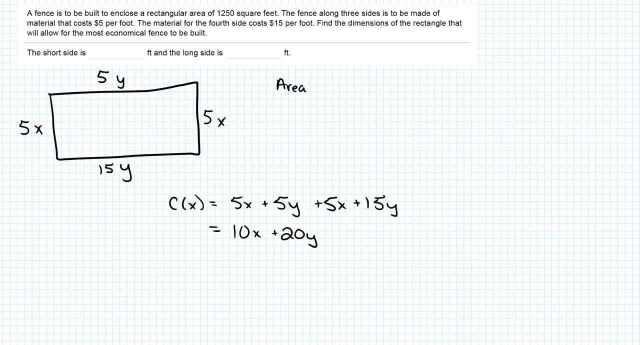 Well, they told us that the area equals 1250 feet, And so X times Y equals 1250.. So if I want to solve that for Y, Y equals 1250 over X, which is the same thing as 1250X to the negative 1.. 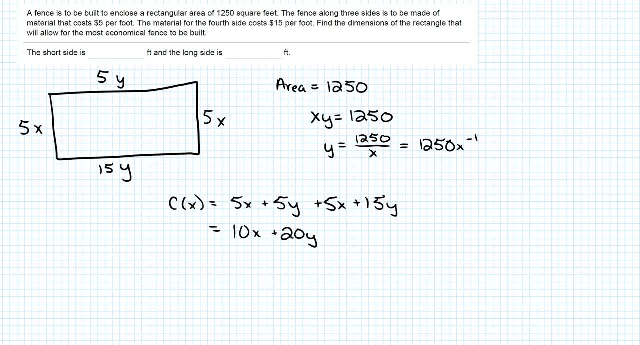 And having that exponent like that instead of the X in the denominator is going to make it easier for us to take that derivative. So we have 10X plus 20.. But instead of Y I'm going to plug in this 1250X to the negative 1.. 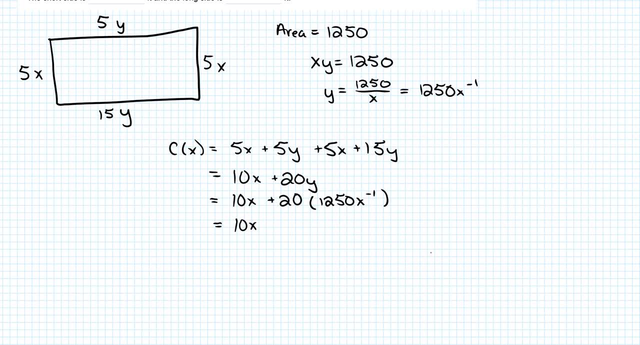 Now, if I simplify that, I'm going to get 10X, And if you do 20 times 1250 in your calculator, you're going to get 25,000X to the negative 1.. So that's the simplified version of my cost function. So the next step is to take a derivative. 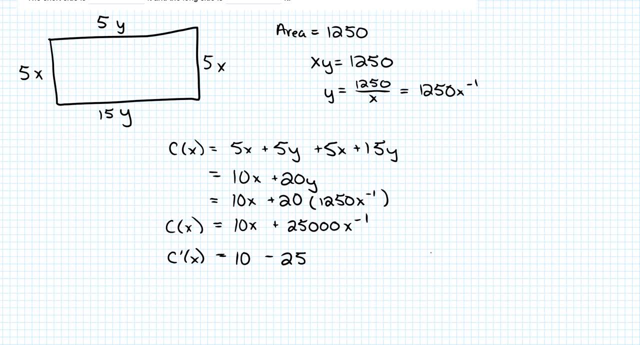 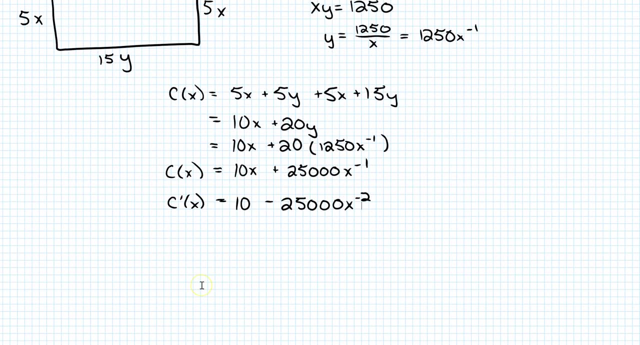 And that's going to give me 10 minus 25,000X to the negative 2.. Then the next step after that is we're going to set our derivative equal to 0. So I have 10 minus 25,000X to the negative. 2 equals 0.. 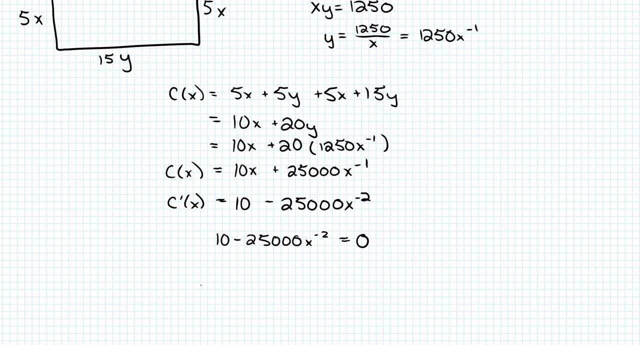 And in the last video I showed you how to get rid of that negative 2 exponent so that we don't have to worry about it, And so that was basically multiplying both sides. So I'm going to divide both sides of my function. times X squared. 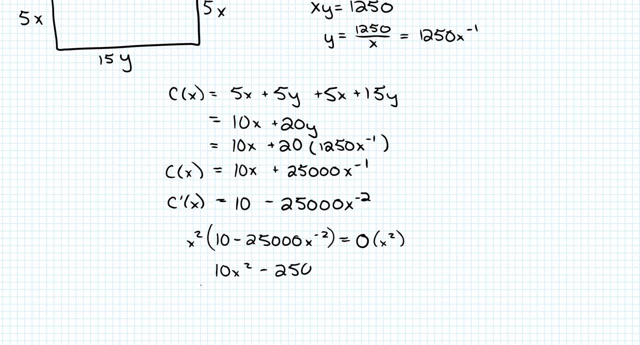 And that gave me 10X squared minus 25,000 equals 0.. Again, that's not crazy voodoo. If you're not sure about that algebra, go back and look at it in the last video. So I've got 10X squared equals 25,000.. 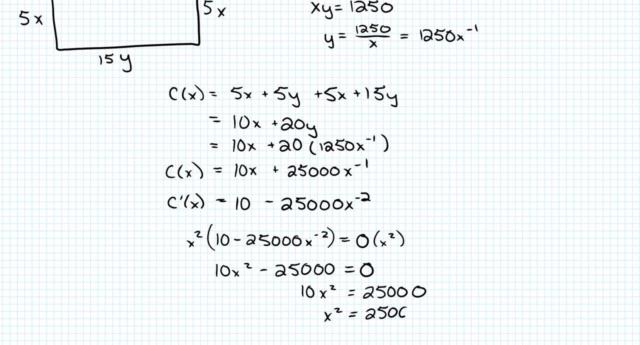 So X squared equals 2,500.. I've just divided both sides by 10.. And now if I do 2,500 and take the square root of that again- you can just do that in your calculator- that's going to give X equals 50.. 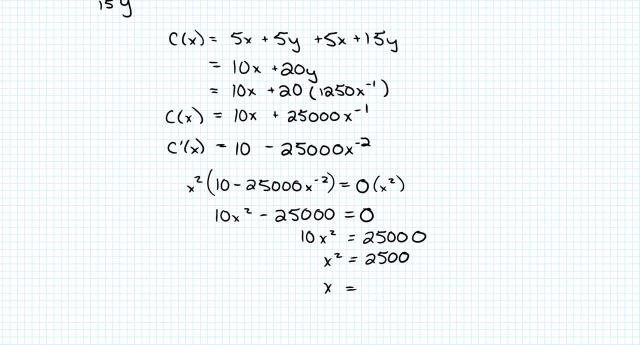 Alright, so X equals 50. And again with the last problem, we talked about how technically the answer is positive and negative 50. But there is no way for a side length to be negative, And so we're just going to stick with the positive answer. 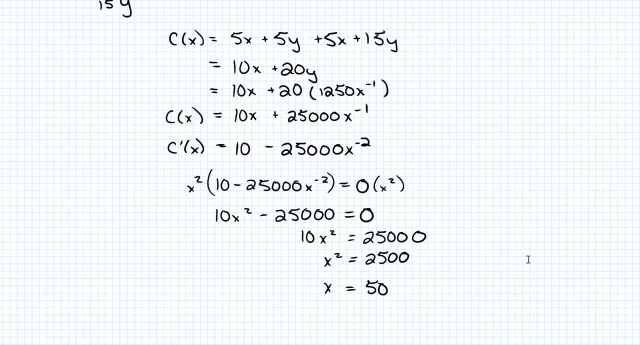 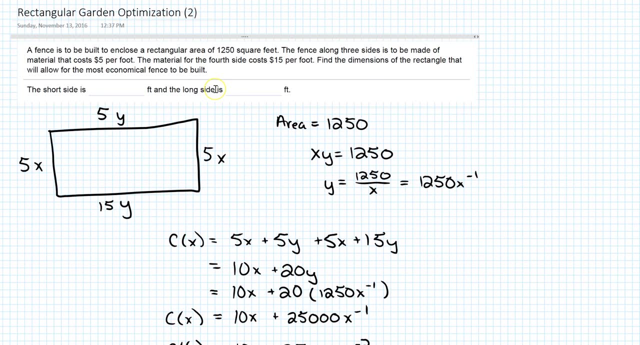 So this is telling me that the X side is 50.. So let's go and look at what the question is asking. The question says the short side and the long side. So I need to figure out what Y is so I can decide. 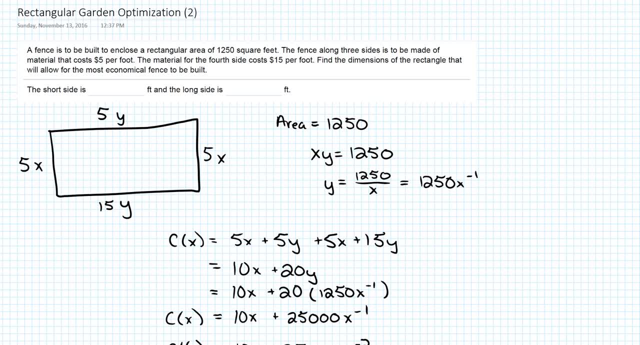 Because I'm not quite sure yet I know what I drew in my picture makes Y look like the long side. But let's figure out what Y equals first. So Y in this case equals 1250 divided by by X. but we just saw that our X equals 50.. 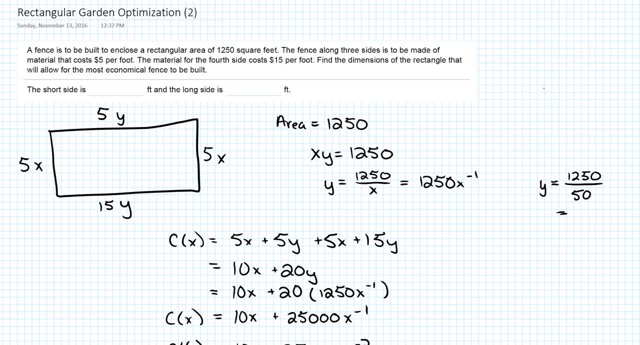 So 1250 divided by 50.. 1250 divided by 50. And that gives us 25.. So actually, once we did the math, it turns out that Y is our shorter side, because 25 is smaller than 50.. 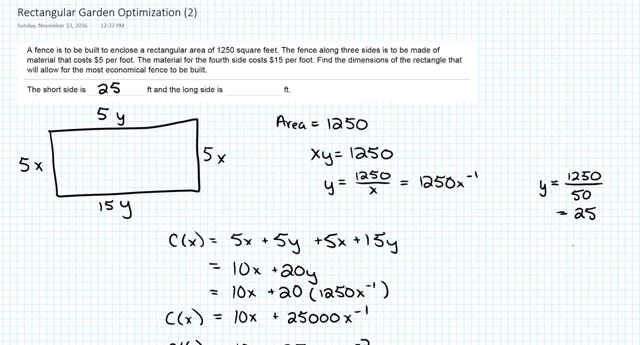 So the length of the short side is 25 and the length of the long side is 50.. And again, if any of that didn't make sense, go back and look at the question again. And again, if any of that didn't make sense, go back and look at the question again.